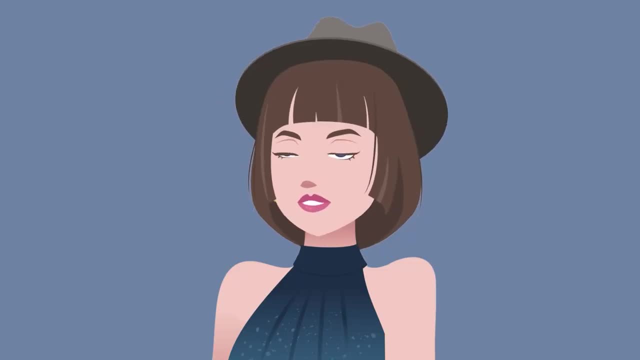 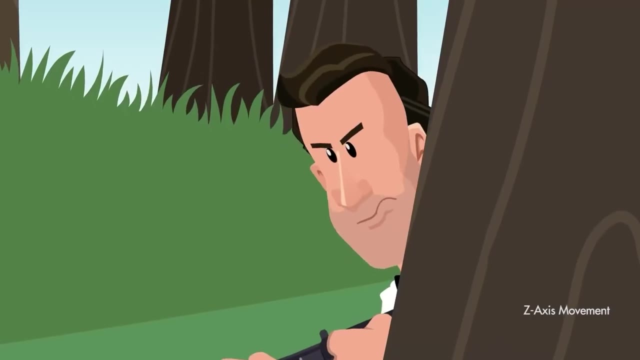 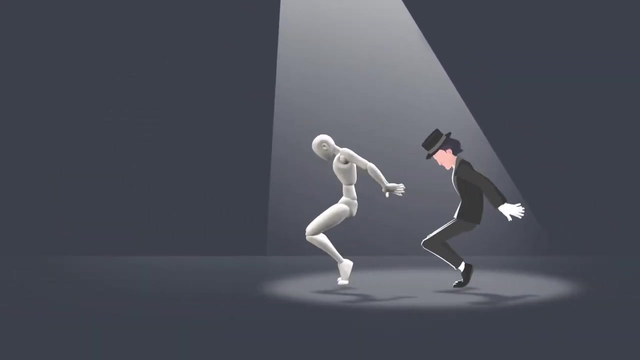 If you have ever wanted to animate but found it hard due to your inexperience, or if you're an animator who wants an easy method to go about your animation, whether for a quick conceptualization of your animation or for a final project, you might want to sit down and discover Cartoon. 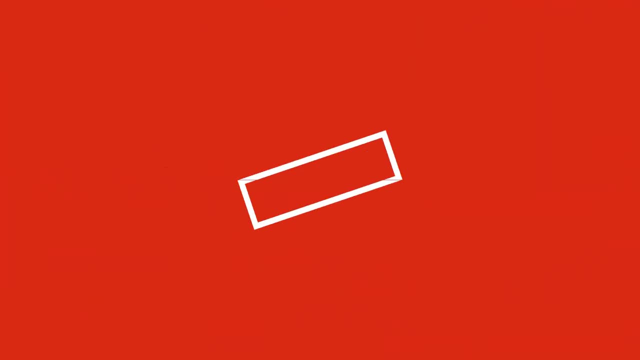 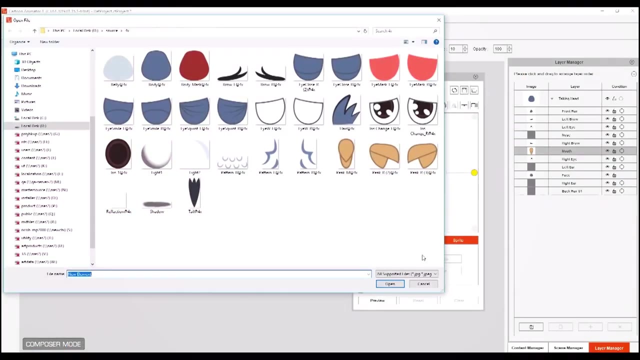 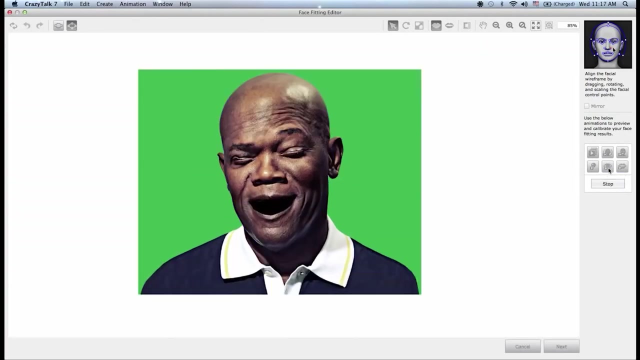 Animator 4 with us through this video. Cartoon Animator 4, formerly known as Crazy Talk Animator, is a 2D animation software developed by Reallusion, the sponsor of our video today. Cartoon Animator is the type of software that takes laymen and professionals in animation. 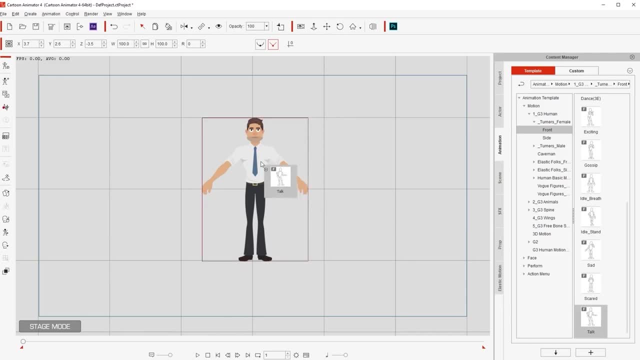 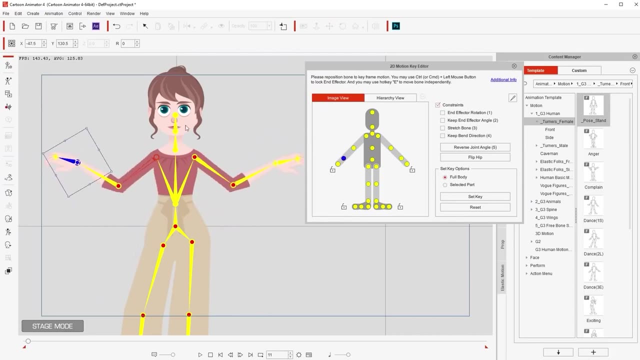 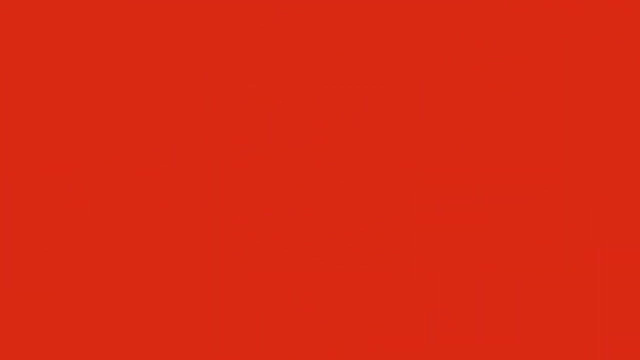 into consideration alike. The software will help you animate your 2D assets by providing you with an incredibly powerful set of tools and features to help you bring your vision to life with ease, no matter your skill level. Upon opening the software, you will be met with a white, clean-looking user interface. 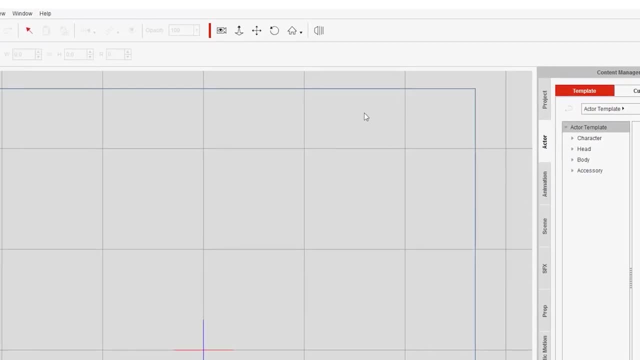 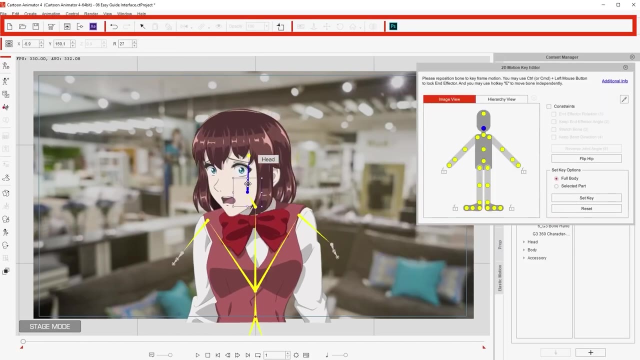 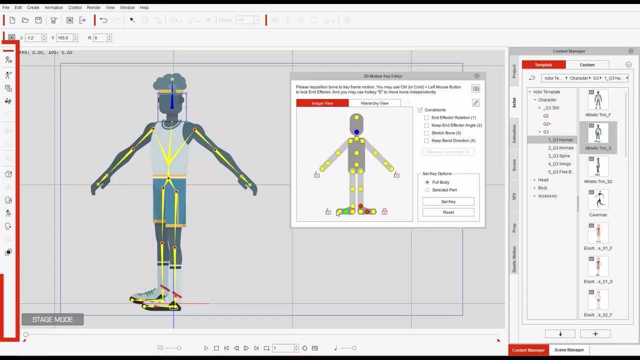 The software is designed in a similar way to most 2D animation software, so if you're familiar with those, you'll feel right at home. You have the menu bar at the very top and three panels, one right underneath the menu bar, one on the left, with quick actions such as compose. 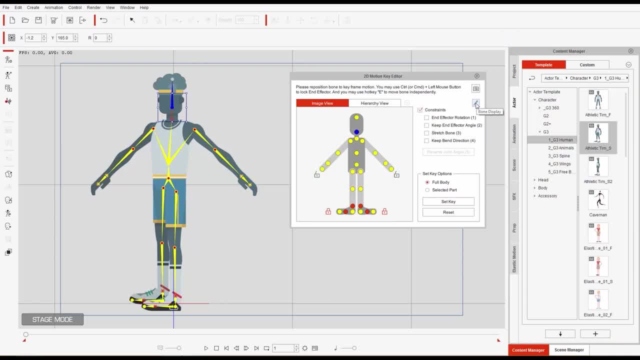 create a character and create media, and the panel on the right, the content manager, where you can find a library of the content. you add different kinds of pre-made animations, special effects and so many other features. On the bottom is where you. 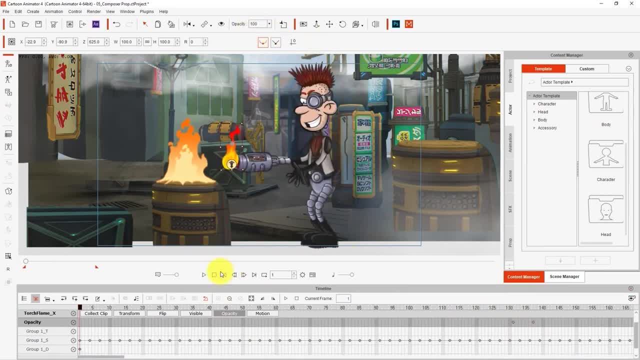 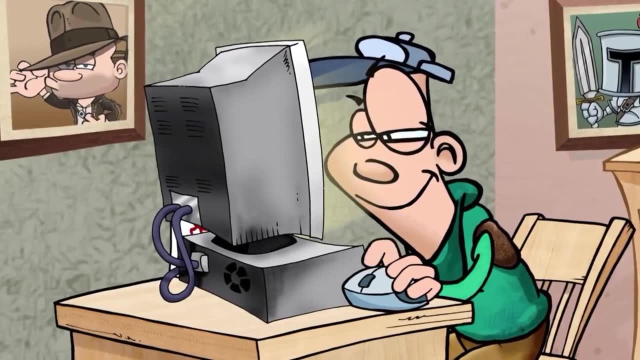 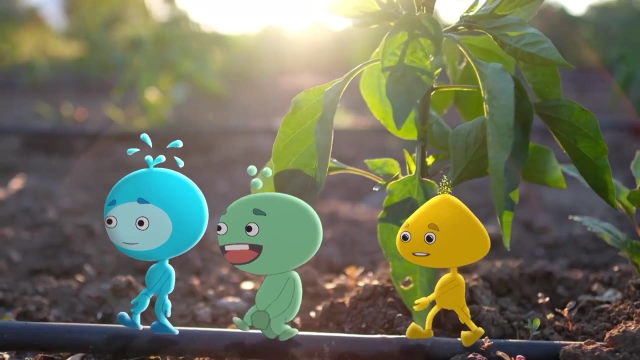 can find the timeline if you choose to show it alongside the playback options. Now let's get to the exciting stuff. What can this software actually do? This software can do much more than we're going to mention here, but we compiled a list of the most interesting. 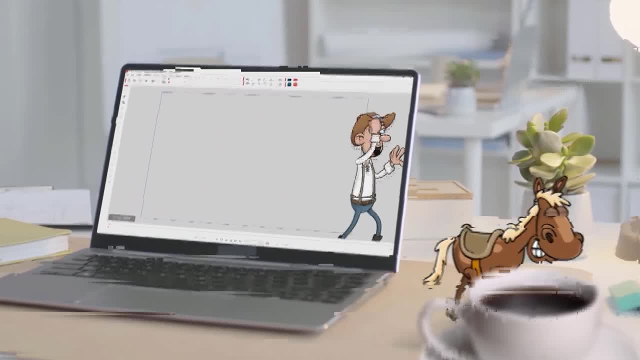 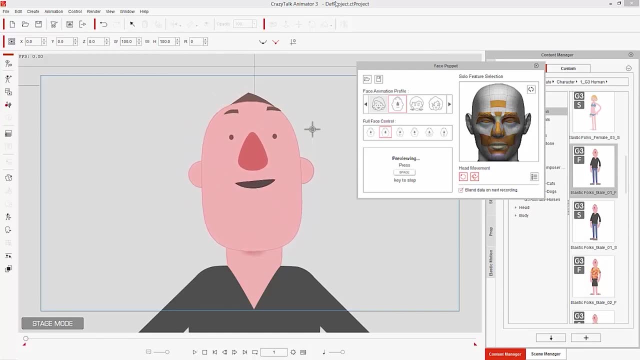 and exciting features the software has. So let's dive in Face Puppet. Animating faces and expressions has never been easier. Cartoon Animator uses advanced technology called Generation 3 and G3 360 to make animating faces and expressions a simpler process. All you would need to have a fully rotating head is a couple of 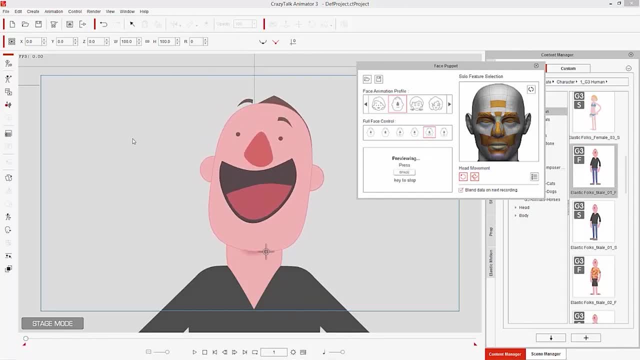 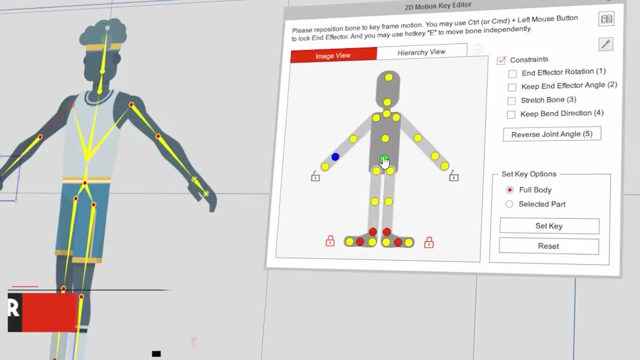 sprites and you're good to go. Cartoon Animator can also help you generate lip syncing, but if you like it, you can still edit it and do it manually. 2D Motion Key Editor. Cartoon Animator 4 now makes it easy for you to animate body movements. 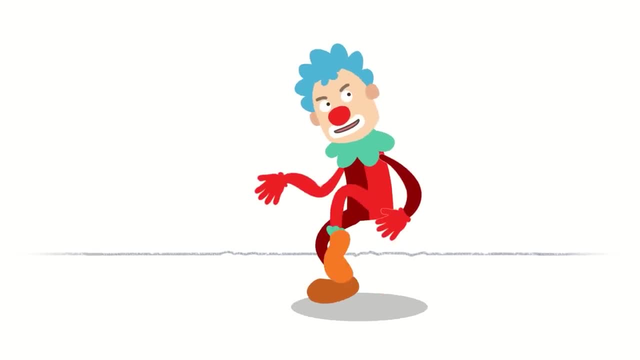 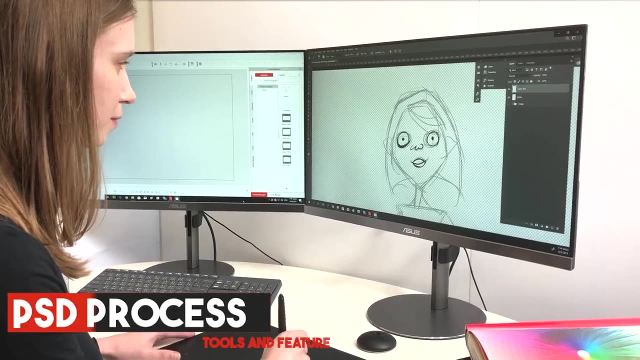 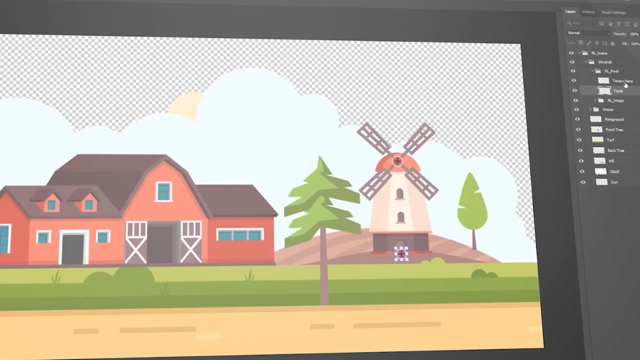 It facilitates setting or key modifying in motion-related tracks by using a more intuitive and interactive interface. PSD Process Cartoon Animator 4 is designed in an intuitive way for everyone to use. Are you a graphic designer who doesn't wish to learn complicated graphics? If you want to learn more about graphics. 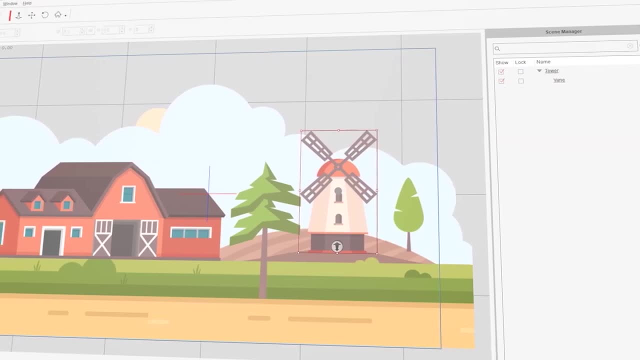 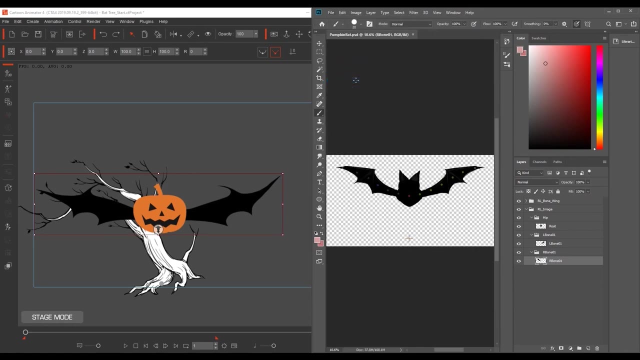 you can use a little more advanced and sophisticated rigging processes, but rely on an Adobe product to make your designs and don't wish to make them elsewhere. Well, Cartoon Animator 4 breaks any walls between Photoshop and many other 2D graphics editors to. 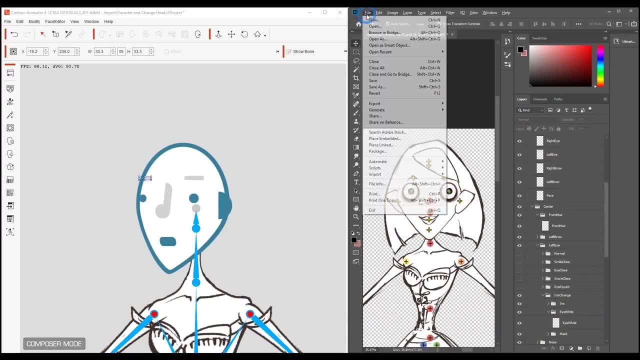 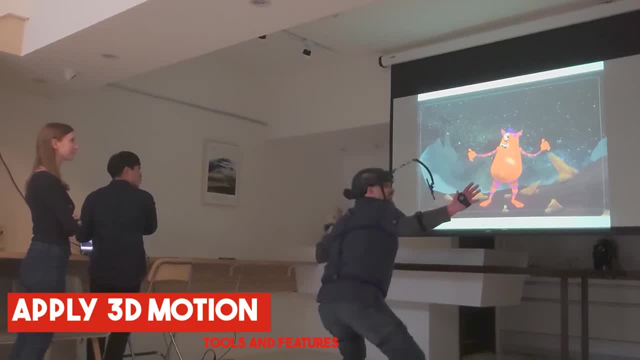 help you very easily go back and forth between the two software and seamlessly play around with animating your creations, even if you're at the sketching stage. 3D Motion: Apply 3D Motion. Imagine you could animate your 2D characters using your body's animation. 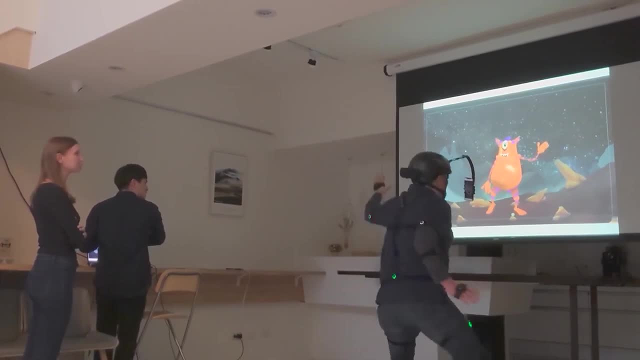 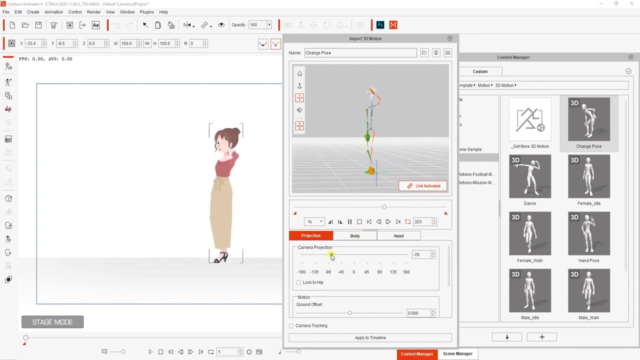 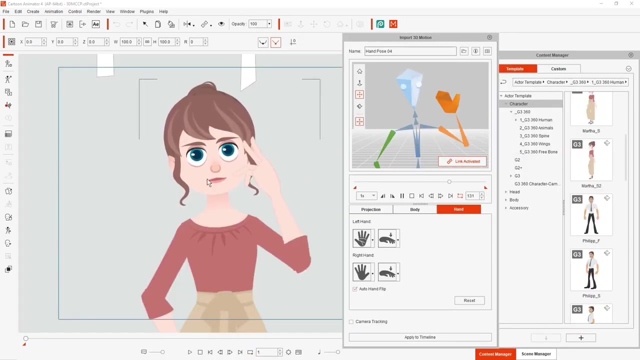 Instead of having to animate the character frame by frame. well, you don't have to imagine anymore. Cartoon Animator 4 allows you to use motion capture technology to animate your characters. You can set up any drawing character or creature as a live digital puppet with real-time animation. 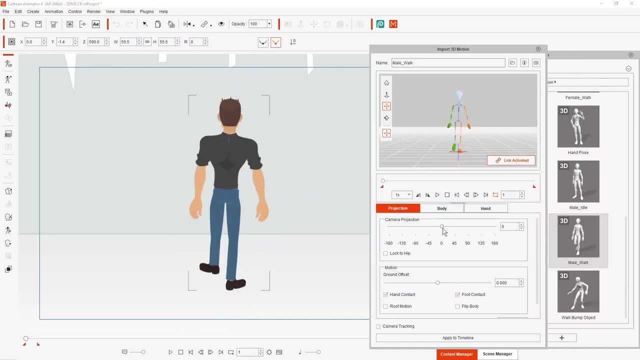 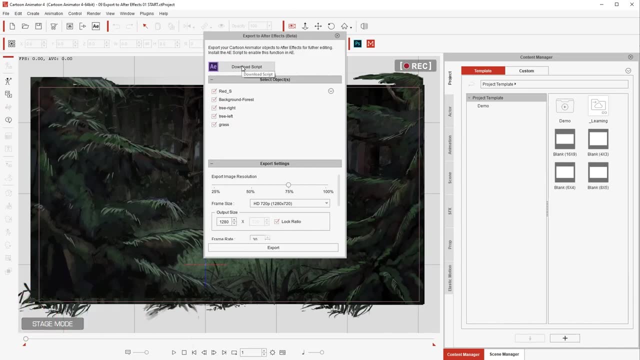 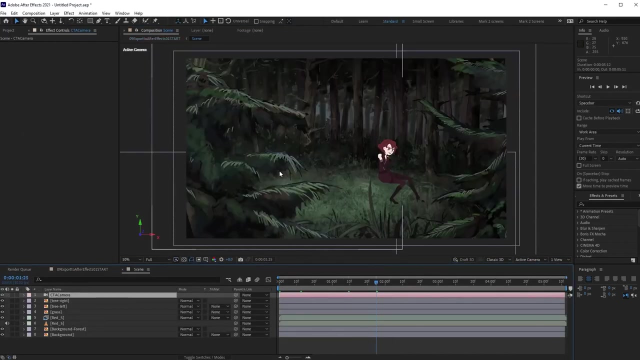 This can be a game-changer in the making of animated shows and movies. Export Video Compositing In Cartoon Animator 4, it is possible to export an object as a video and then import it into After Effects and composite it there. The process is very quick and seamless. 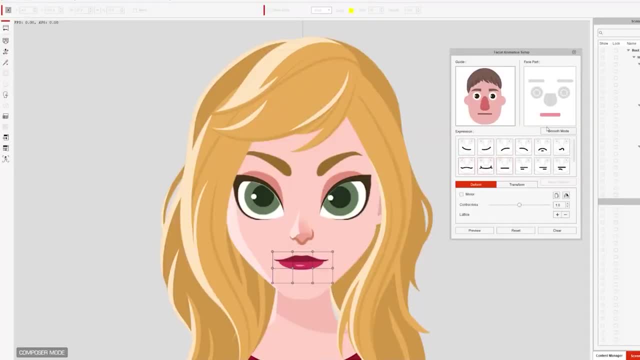 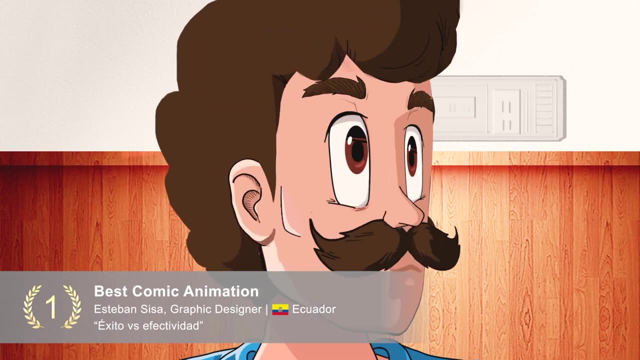 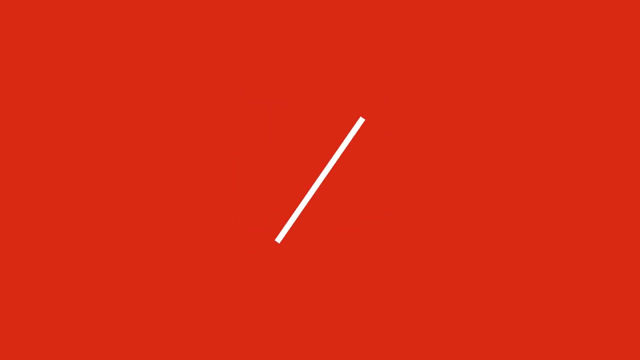 Features. These features are amazing, and we haven't even cited half of them. Feel free to check Cartoon Animator's website for more information on the many tools and features the software has. Okay, now let's talk pros and cons. Pros and Cons. Features: Apart from having great features, Cartoon Animator 4,. 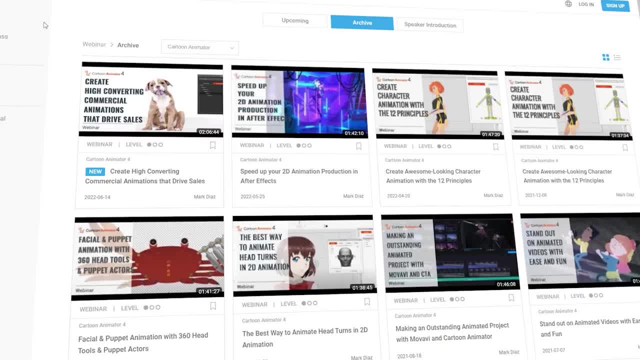 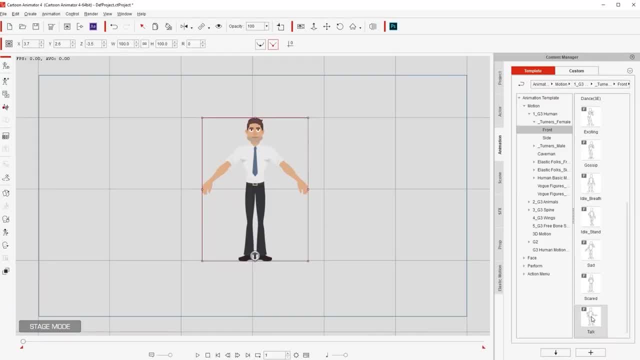 provides you with an amazing array of free resources, one of which is their free webinar, which will be hosted in June and July 2022, featuring Mark Diaz. Another great feature about the software is the availability of free and paid assets to use in. 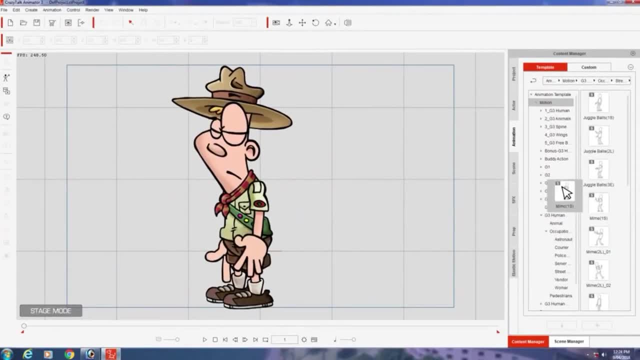 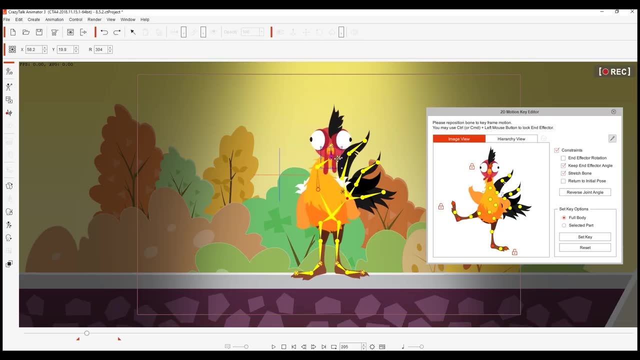 your animation. So if you're not an artist but want to make a quick animation for a presentation or an explainer video, you can do that with the free stuff And if you like what you see, you can pay for more. Don't like the pre-made characters you see. 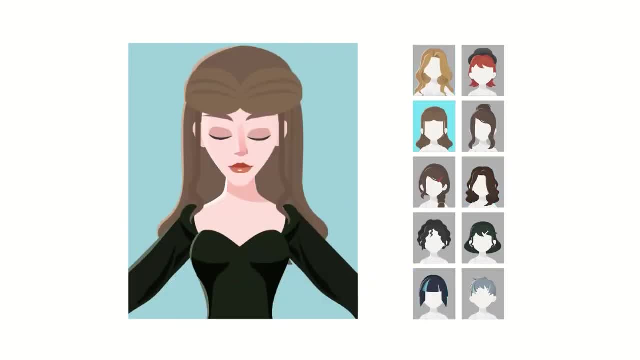 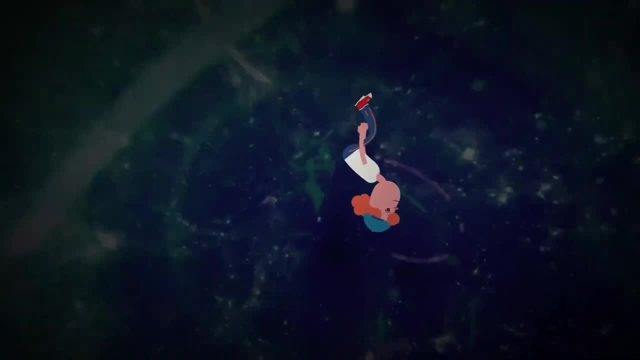 You can assemble one to fit your vision using the actor's function. All these features make Cartoon Animator a great tool for those who know very little about animation but still want to animate. Cartoon Animator 4 is really powerful and versatile, but it's not quite the. 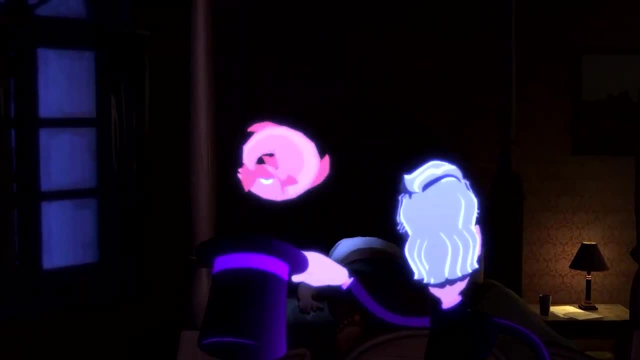 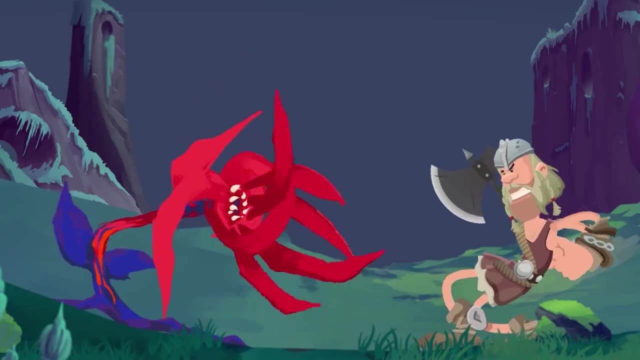 quote-unquote- professional and industry-standard animation tool. It's not the place where you can both create and animate your characters from scratch. You can easily import the assets from a PSD editor and seamlessly jump between the two software. Well, sure, of course. 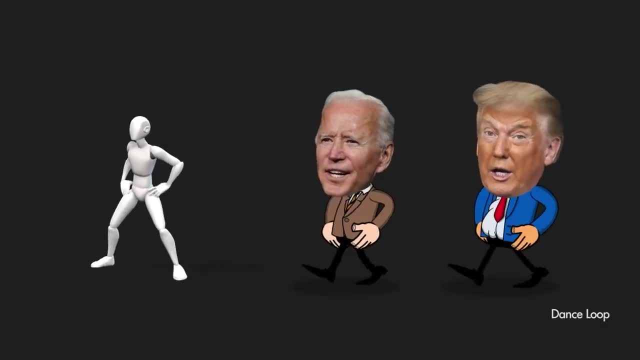 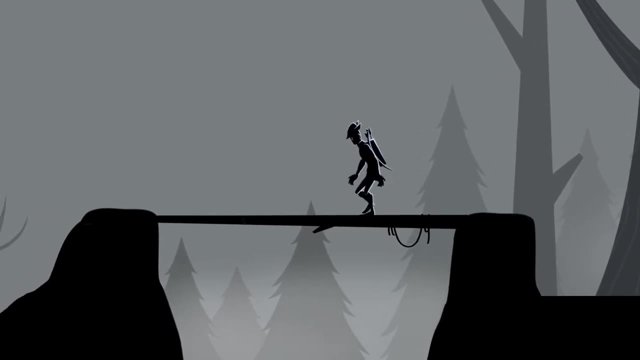 But in that case you have to know how to use both software and you cannot make an animation from start to finish, like sketching, drawing and coloring included, just by relying on Cartoon Animator 4.. So if you're looking to meet the criteria of the industry, Cartoon Animator 4- 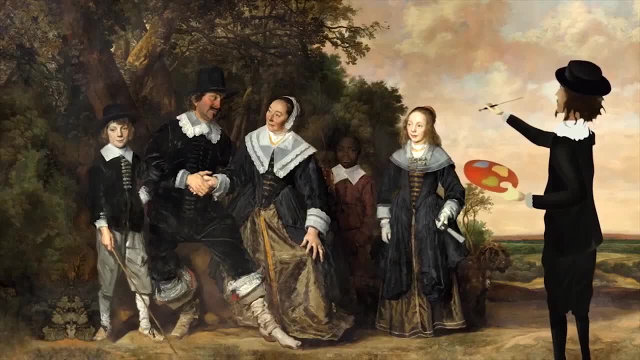 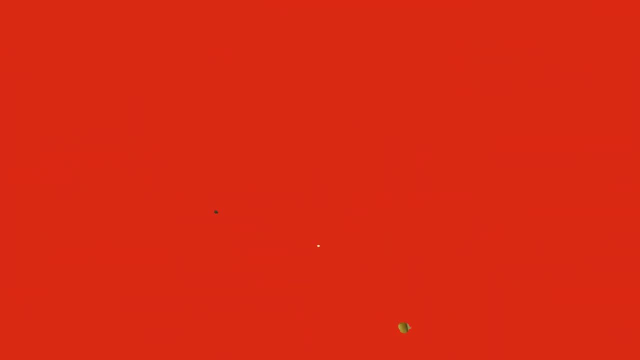 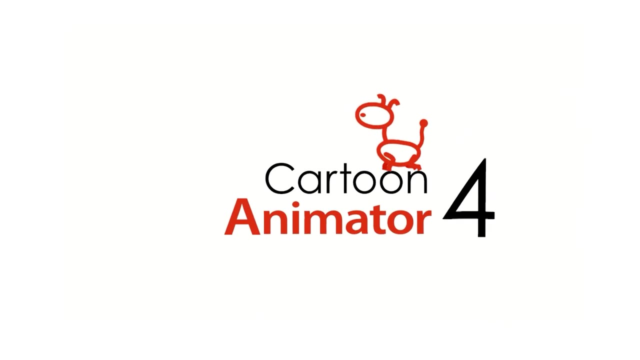 is not the software for you, But if you're a hobbyist content creator or a professional freelancer, you can expect this software to deliver more than we could fit in this video. Okay, now that you know how much of an amazing software Cartoon Animator is, let's show you a quick. 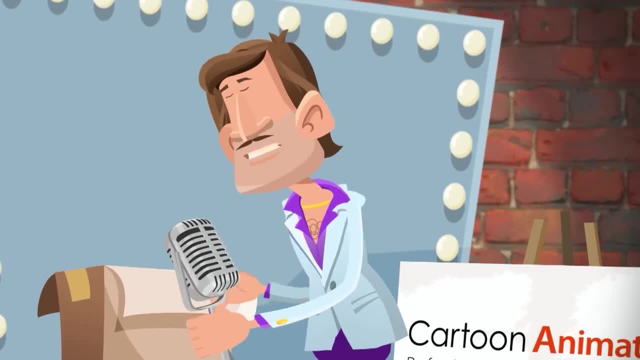 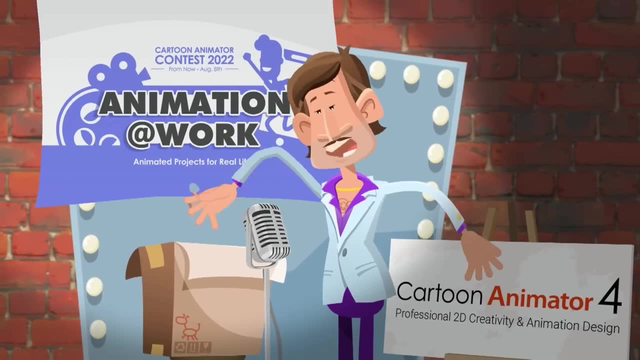 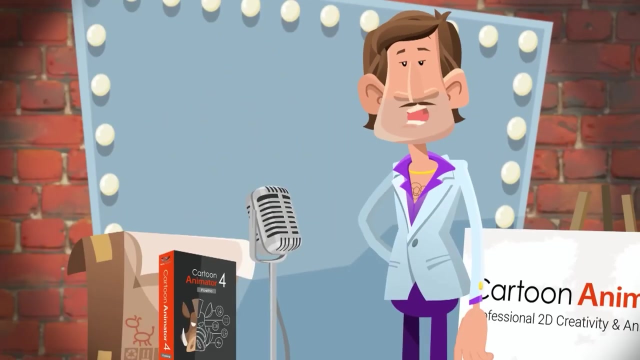 way to get the software for free for two months. A Cartoon Animator contest is being held, and no, you don't even have to participate. All you have to do is share the contest's website and tada you get a two-month free trial. Now what happens if you actually join the contest? 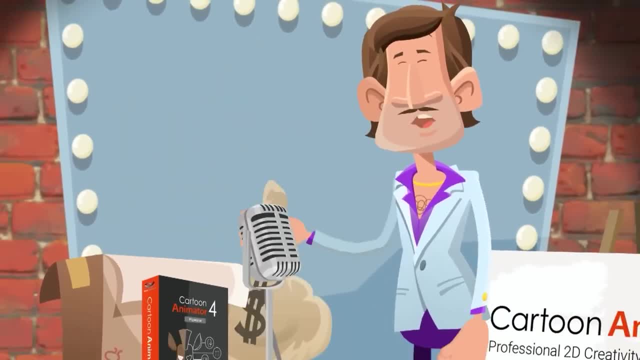 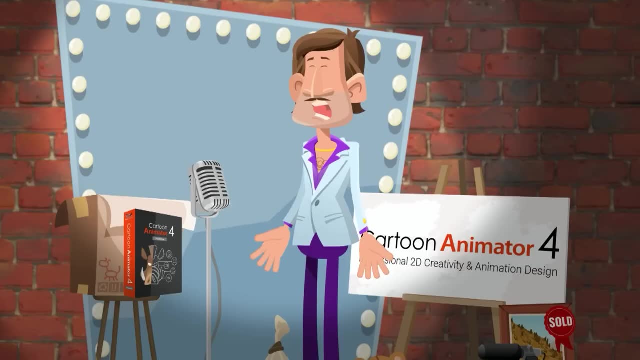 Well, you might get amazing cash and sponsored prizes. The rules for the contest are simple. You must submit your entry between May 13th to August 8th 2022,, of course, This year, The winner will be announced on August 23rd 2022. 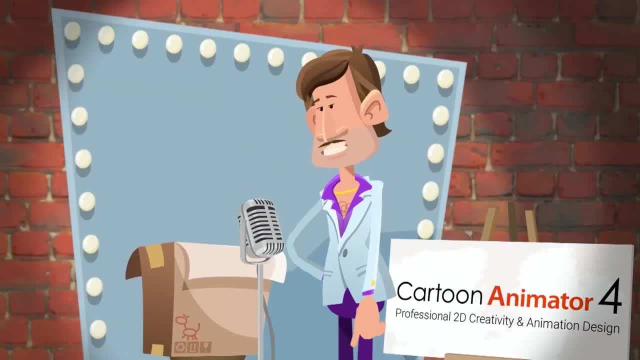 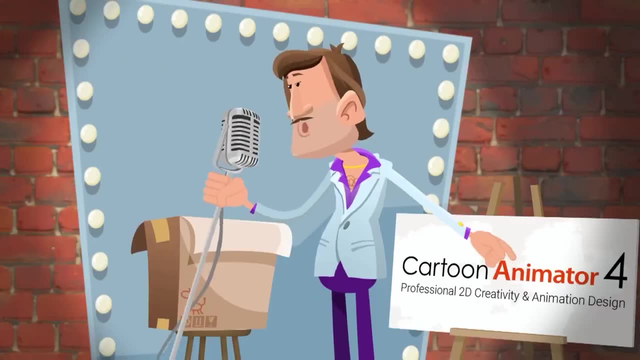 But what do actually need to submit? You must choose a category and create a 2D animation video made with Cartoon Animator Pro or Pipeline. Make sure to have a creation that matches the category. at least if you can do it, Then don't just treat those wonks scream If you receive a win at first. 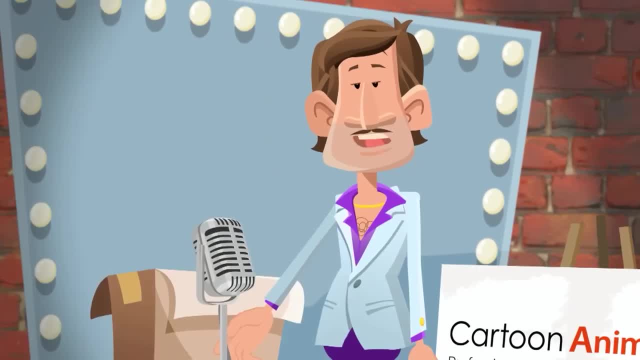 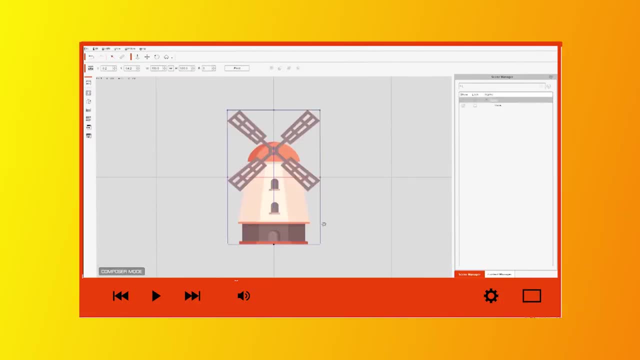 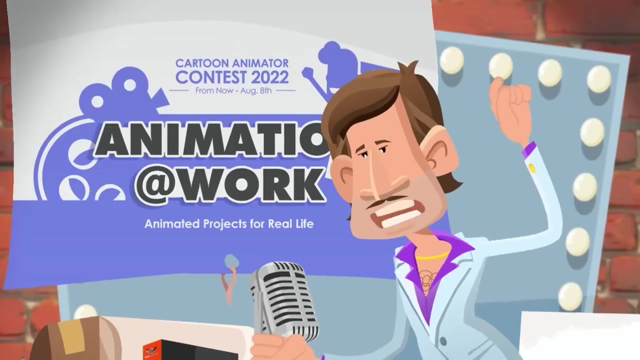 description and be original. You then upload your final video entry and a speedpaint video on YouTube or Vimeo: a work-in-progress video of the animation you made, which must contain key steps on how you made the animation with Cartoon Animator. Your entry must have the contest logo. 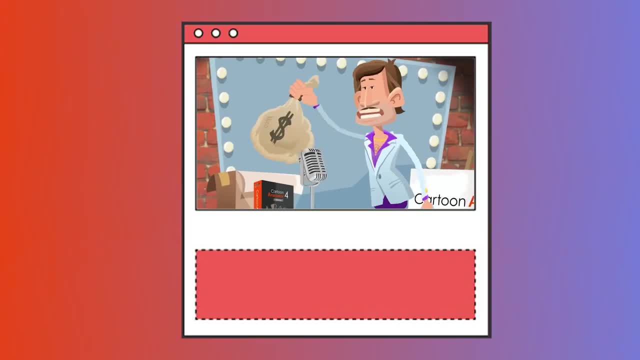 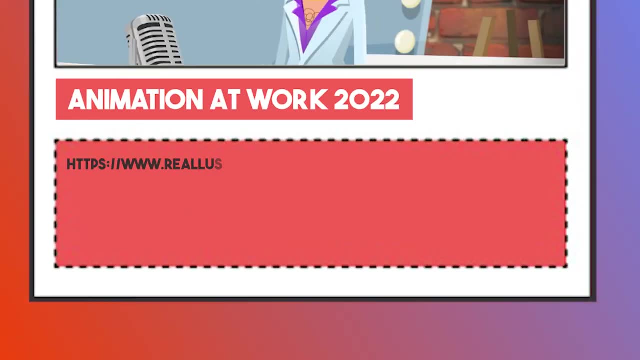 at the end for at least three seconds. The title of your entry must begin with the text Animation at Work 2022.. The video description of the entry must include Cartoon Animator link appearing on the screen right now, And of course, we'll leave it in the description too. 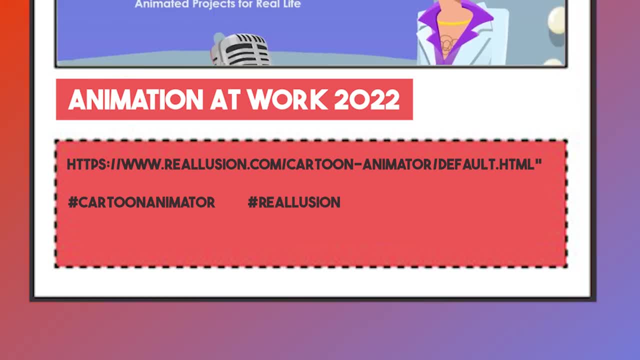 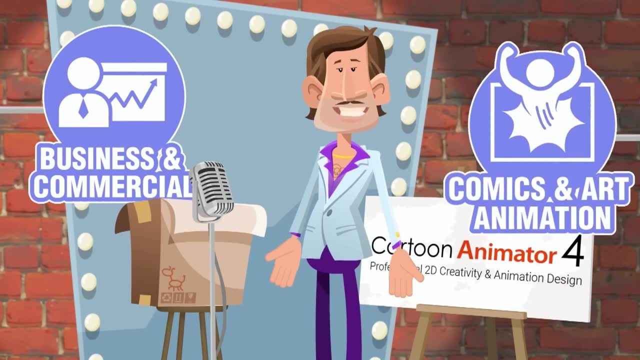 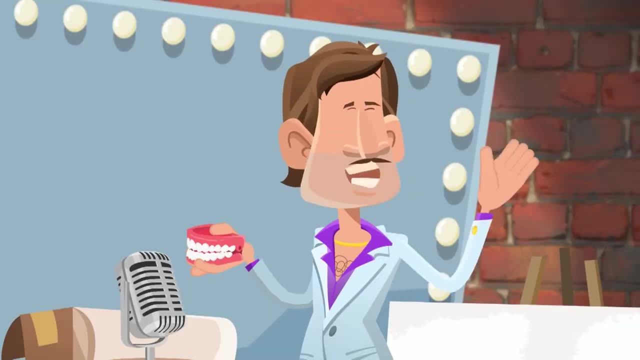 Descriptions need to include these hashtags. We have hashtag Cartoon Animator and hashtag Reallusion. The categories of the contest are Business and Commercial, Comic and Art, Education and Vertical Short. Okay, you might be wondering why even join. Well, 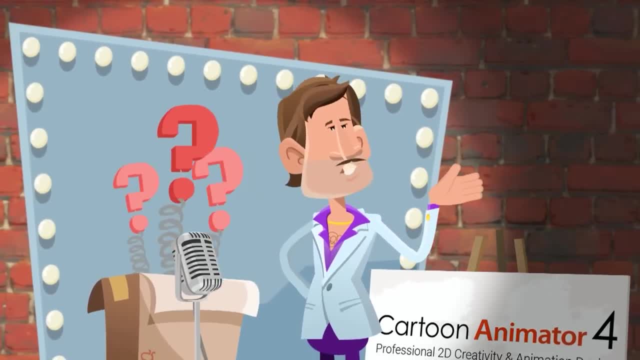 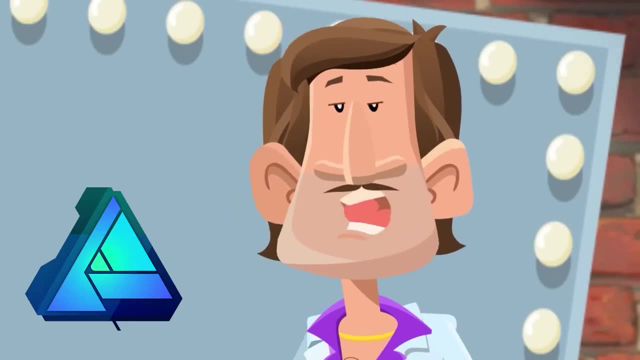 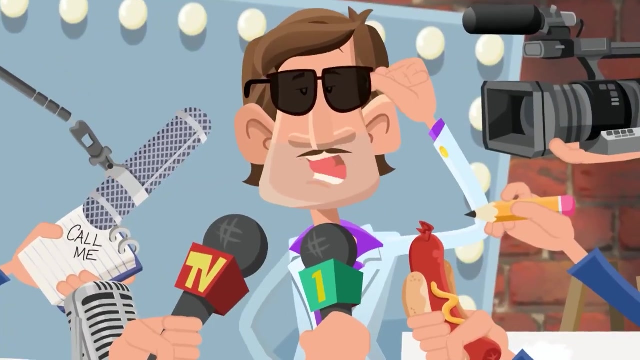 let me tell you, the prizes are amazing. You can win cash prizes alongside another type of prize. You can win powerful software such as Affinity Designer, Magix, Vegas Pro and even one of XP-Pen's amazing tablets. In addition, winners will also have a chance to be promoted as content developers. 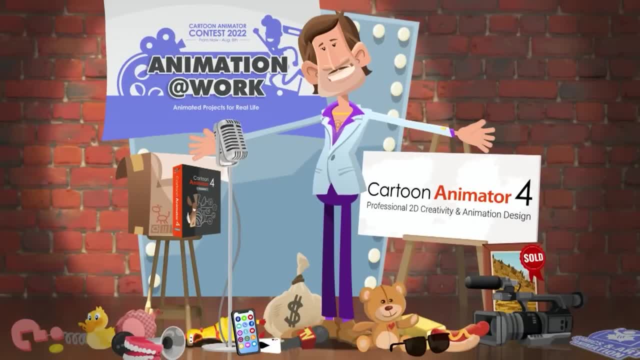 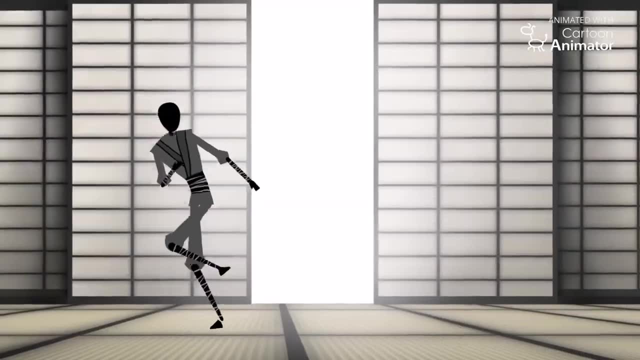 and showcase partners. For more information about the contest rules, prizes and categories, make sure to visit the contest page. We'll be putting a link in the description below And if you're interested in joining the contest, please do so. Well, we reached the end of our video. We hope you enjoyed it and found it fun. Comment below. 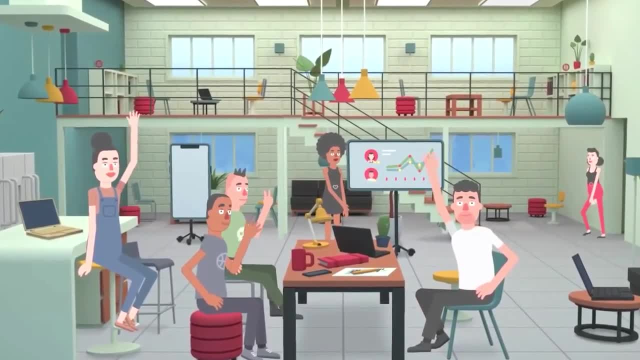 if you think that we've missed something or if you have any other suggestions. Thank you for watching as always and see you next time.